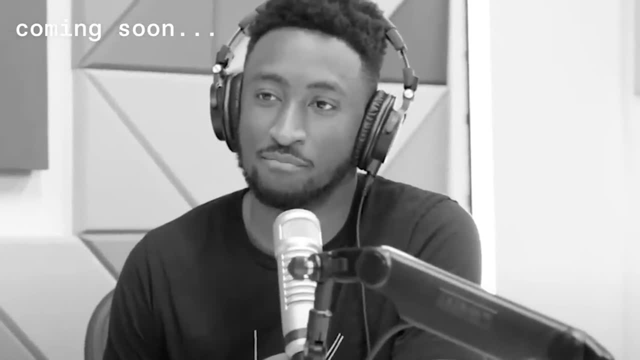 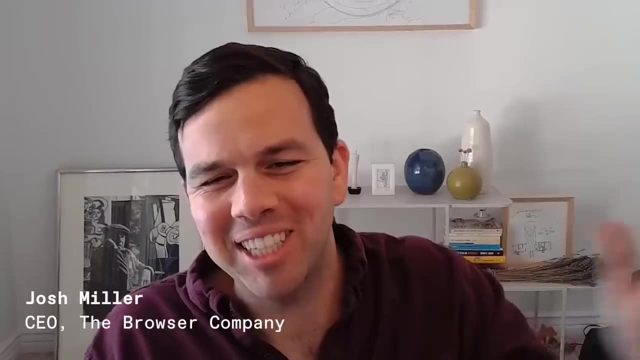 yeah, is this one of those things that's eventually going to get eaten by a major existing browser? no, no, no, no. it has, honestly a ton of different features that i don't even fully utilize. hi, i'm john. i'm the ceo of a startup that just got its product reviewed by mkbhd. 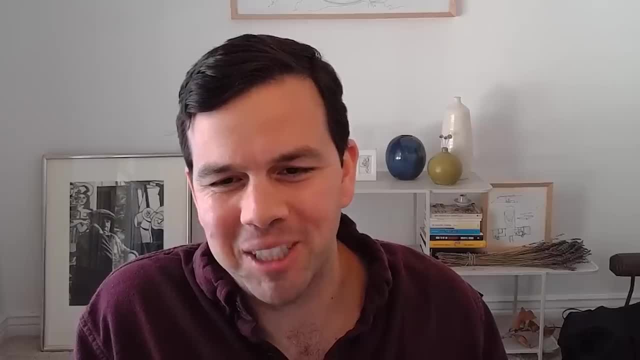 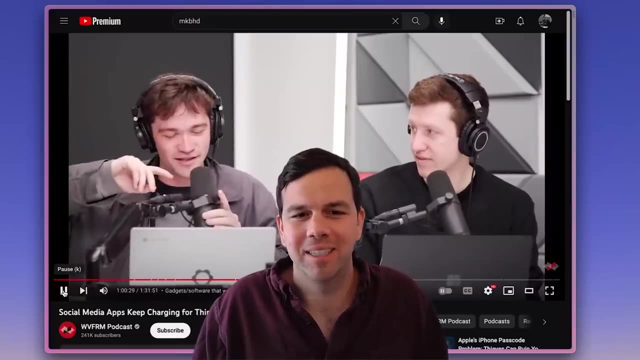 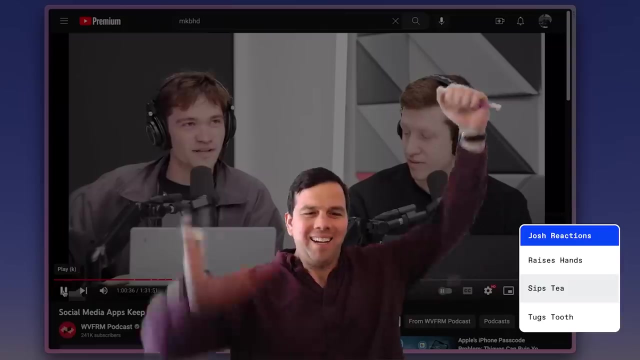 or so i'm told on his podcast, kind of nervous about to watch this live. um, the piece of tech that i have been enjoying because i have not bought anything in like 17 years. um, i, it's a piece of software. it's called arc browser. let's go, that's awesome, that's wild. 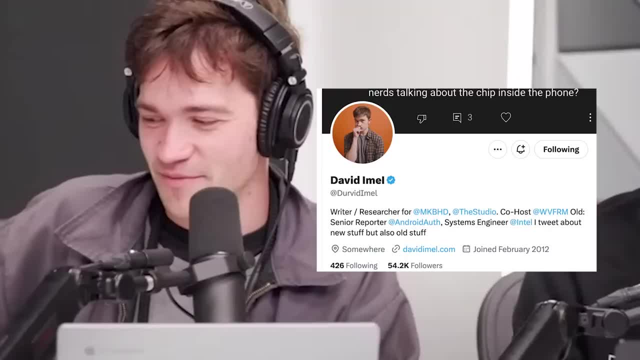 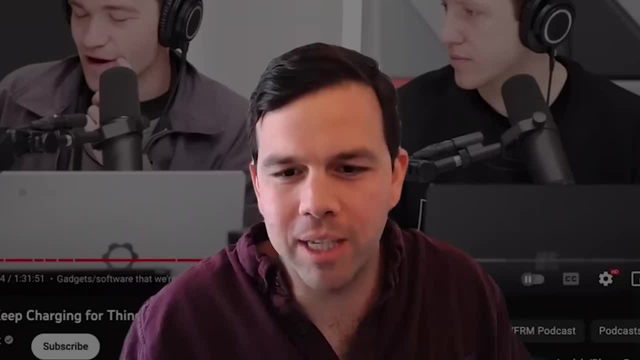 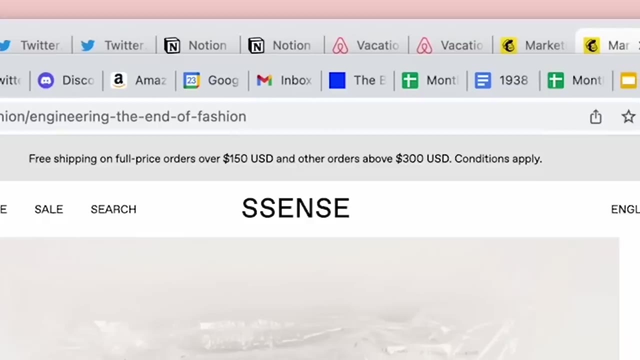 i love this guy. um, you may have heard of it recently in the tech community- my guy david, i think. community, yeah, so yeah, it's called arc browser. um, it is a bro, did he just say? i heard about this, i was there. that basically is made for people who are really bad at tab management, like 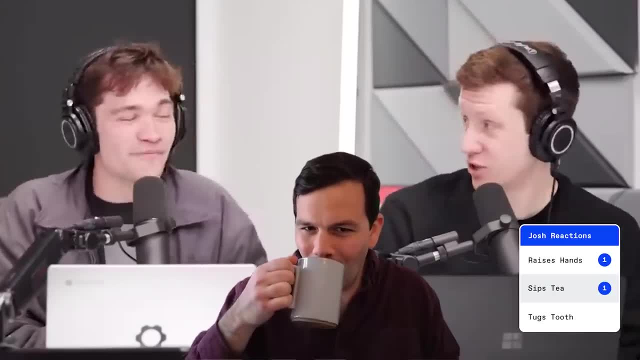 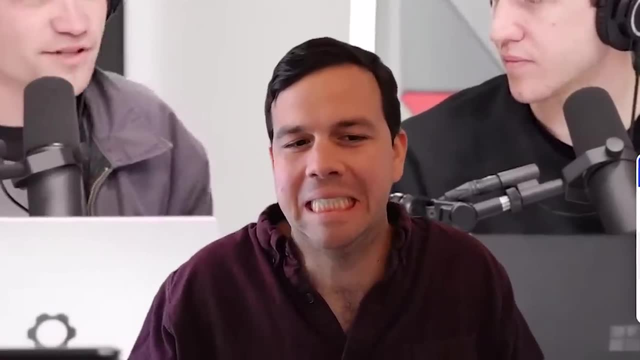 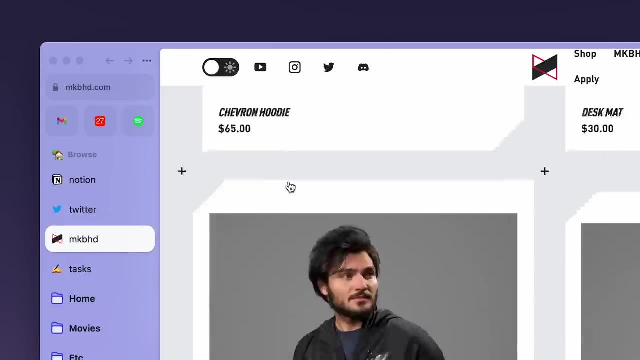 me, um, you're really good at it. well, actually good at it, yes, yes, yes. it has, honestly, a ton of different features that i don't even fully utilize, um, but the main feature is that you have a bunch of pinned tabs that are here that never really go away. okay, and what's cool about them, too, is that you can, like you can, peek. 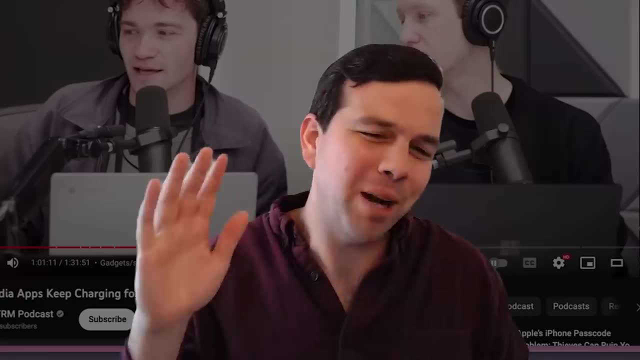 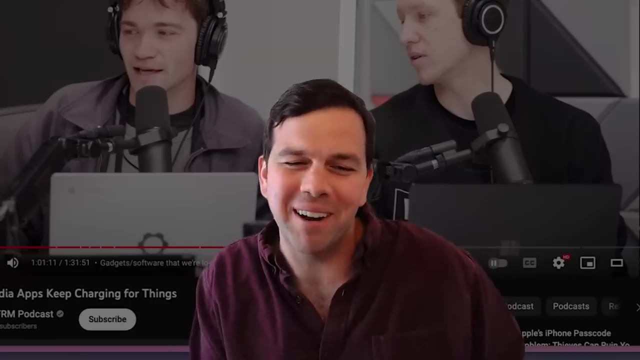 into them and like, okay, when we dreamed about the browser company and arc browser, i don't think you got some pin tabs over here and i don't really use the other features. what was what we were going for? but all right, i'll take it. i'll take it like access things directly, depending on the 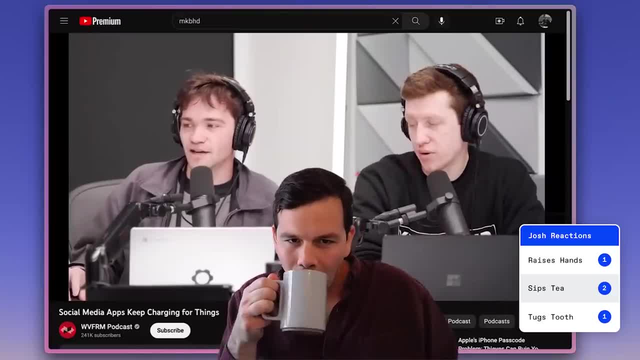 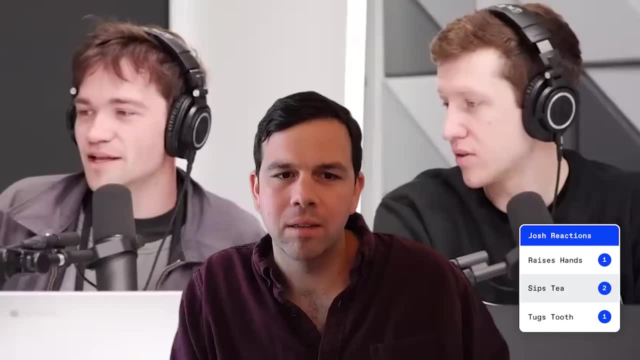 uh, the app that it is or the website that it is, it's a live preview. yeah, a live preview, like his top emails or, yeah, my top emails you can also like. yeah, like in my email. but the main like the main feature that's useful for me is it creates all of these tabs here and within a certain amount of. 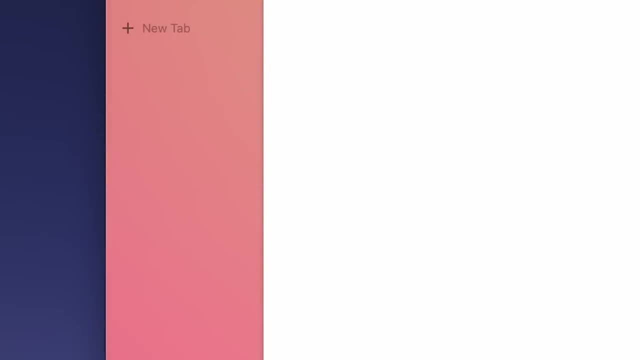 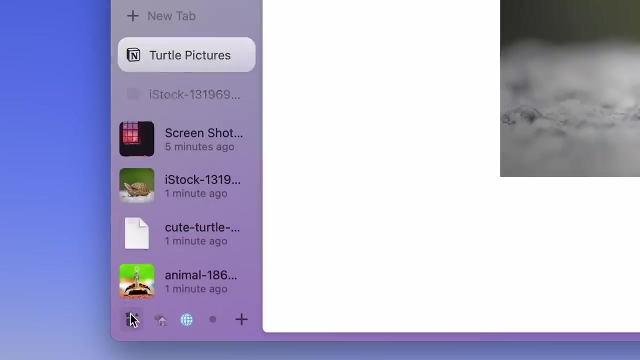 time it erases them, so i have it set for 12 hours. um, there's also all these other features where, like, all of your downloads are right. here. it's really nice, which is really handy, because you can just like drop them into areas. if you need to like drag and drop them into the browser and then you. 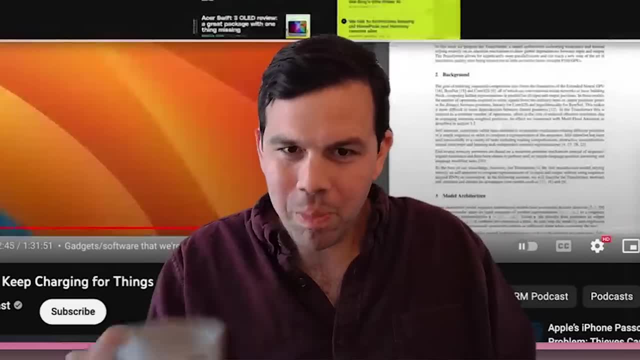 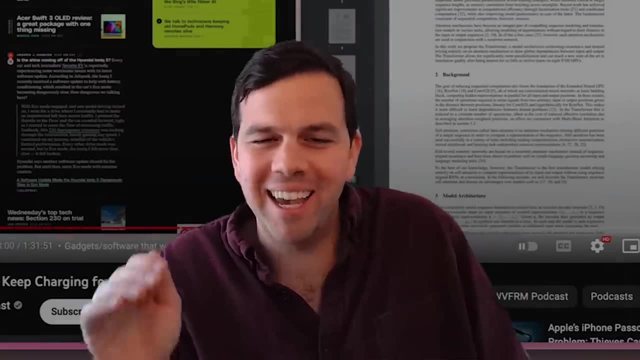 can drag and drop, and then there's like an easel feature where you can like create easels and notes, which i don't even really understand this feature that much. um, i kind of can't believe this was an audio podcast, like if you're listening to this you can say: what is he talking about? all it's missing. 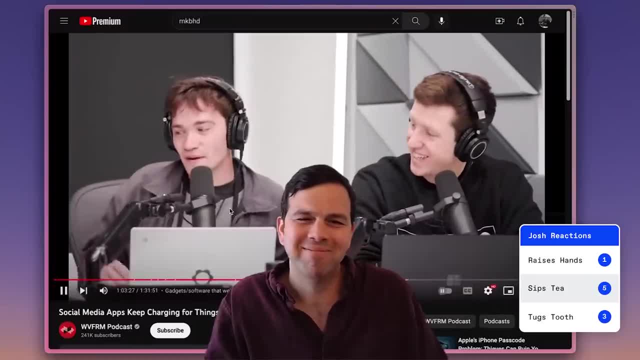 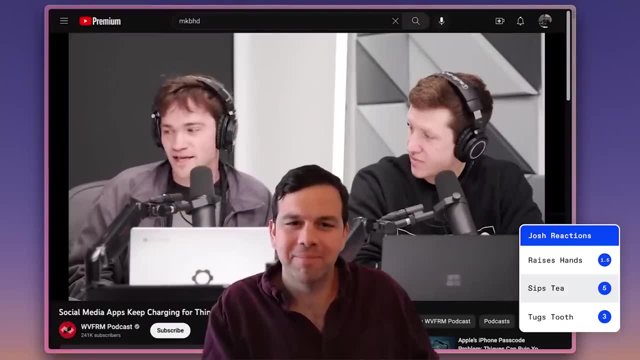 is a chat bot. that's pretty, pretty sick, but they, they up, make major version updates to this like every three days, like they put like huge amounts of work into this and they're like really pressing it and i've switched over to it on pretty much all of my computers. um, yeah, i was gonna say what platform. 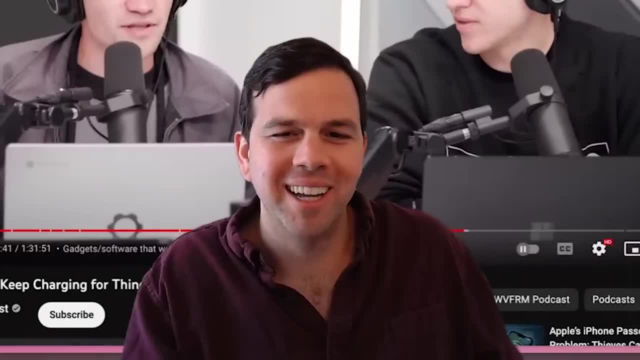 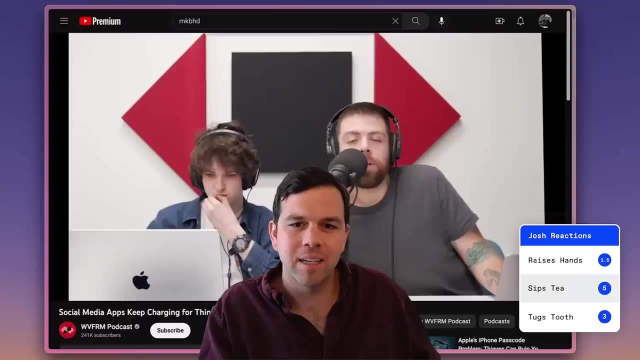 is: uh, it does not right now, totally, so that's only mac os, but they have a. they're building a windows version right now, um, and they're also building a mobile version- the mobile version too. you can follow them on tiktok, and the developers and stuff will like give you updates. 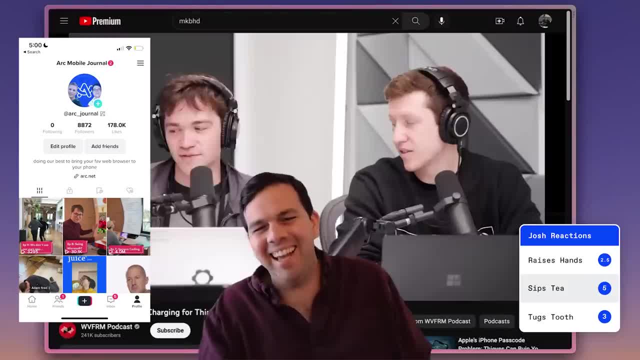 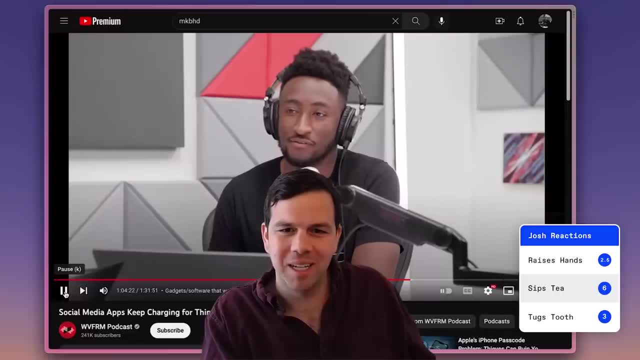 in real time like every couple days. yeah, really clever. yeah, they're very like transparent about. oh, my god, josh, i hope you appreciate that. that's a shout out to you. that's awesome. yeah, is this one of those things that's eventually going to get eaten by a major existing browser, or can they? 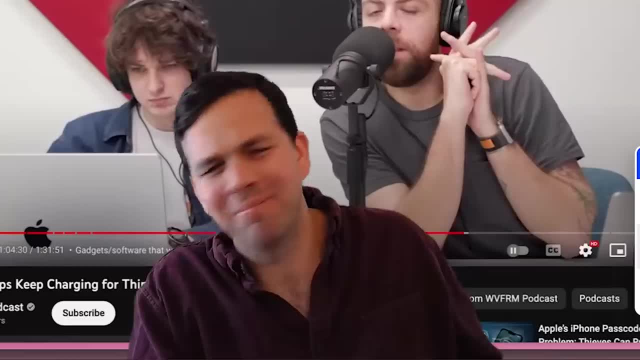 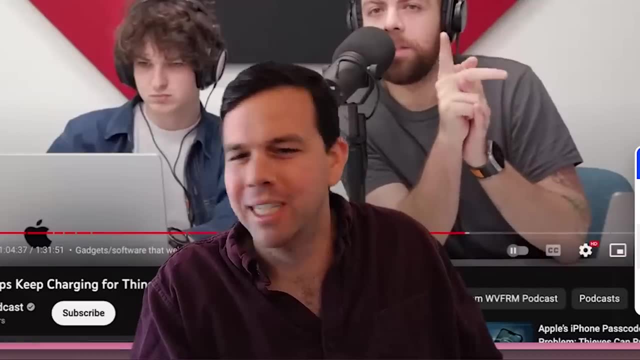 survive and make something. i was wondering that too. i don't think so. i don't think so. there's enough uniqueness here that i think it could be its own thing. yeah, i think i was telling, i think i was telling david this. i think this is what, like chromebooks could have been. it's in the company that's making. it's called the browser. 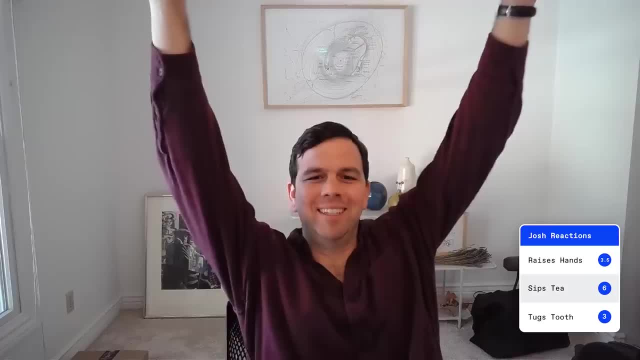 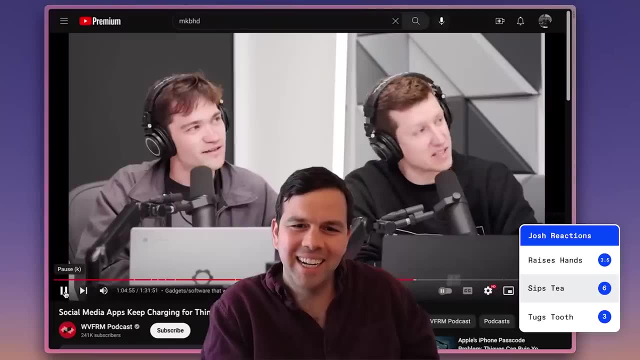 company, which is a great thing, is a good great name, yeah, by the browser company. that's tight, which is very cool. so it's free, it's free, cool, that's. that's awesome. i think it's niche enough that, like i don't know if chrome would benefit fully taking over it, because, like i just mean, 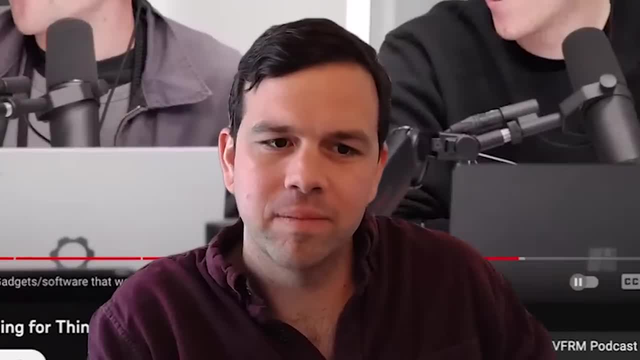 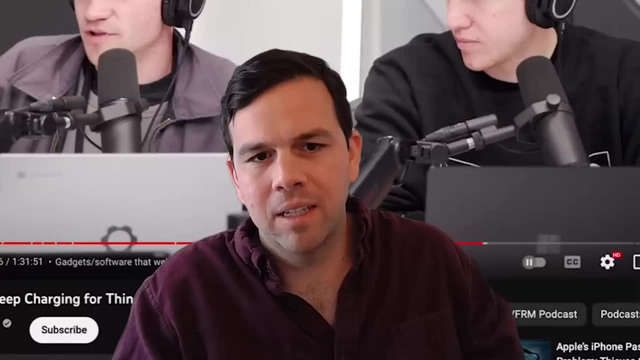 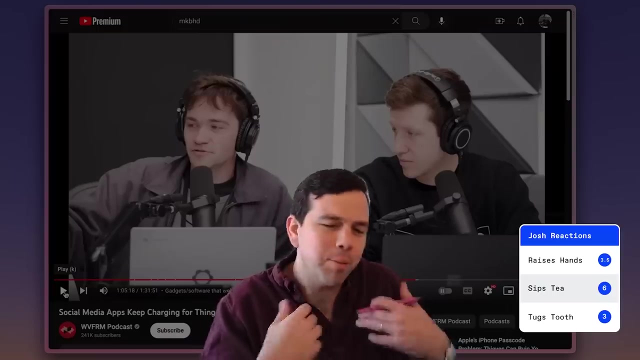 like stealing, unprotected features, yeah, like anyway. yeah, and i have like a bunch of research, uh groups and you can also create these new new folder, new space, like spaces too. oh man, this is a i don't know how to take this because, on one hand, we're very prep. i personally believe i wrote this. 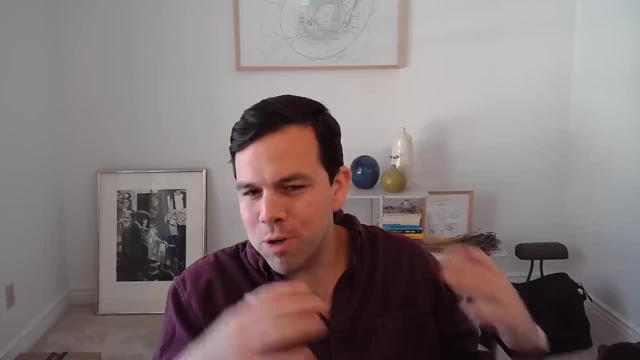 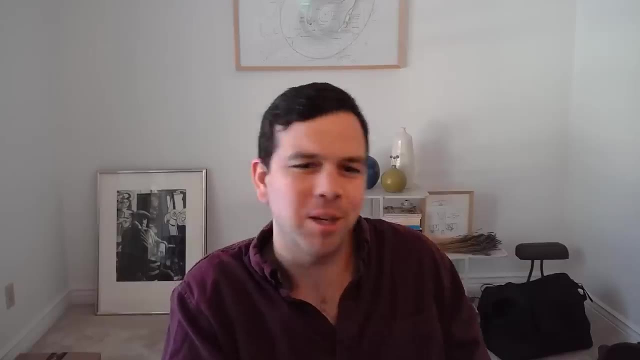 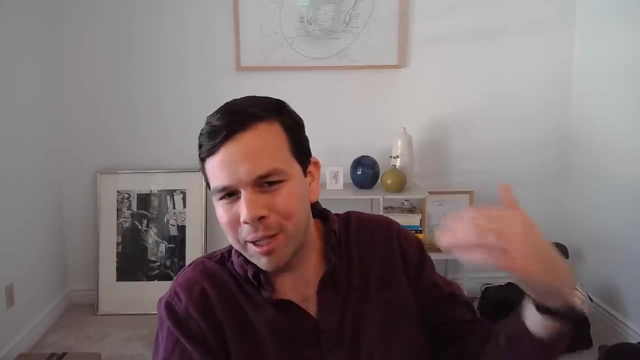 essay a couple months ago that the real transformative pieces of technology almost escape explanation, like how did you explain snapchat the first time you used it? or how did you explain notion? or even the iphone relative to a blackberry. so like on one hand, i kind of love that this guy is struggling so hard to give like a crisp pitch. 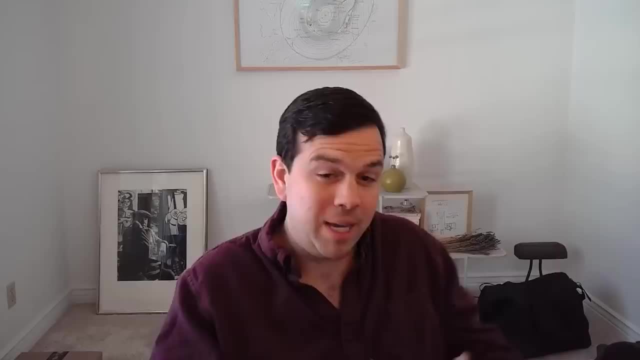 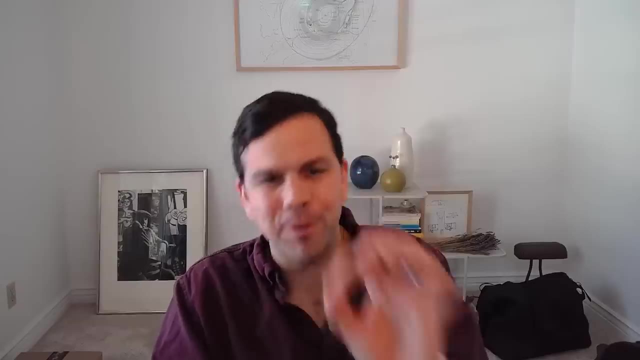 for arc because it means that we probably built something really new because he is so passionate about it. on the other hand, it's like it is pretty painful that like we don't have a crisp focused. this is why arc's awesome. i need this to be multi-platform before i can dedicate my life to it. 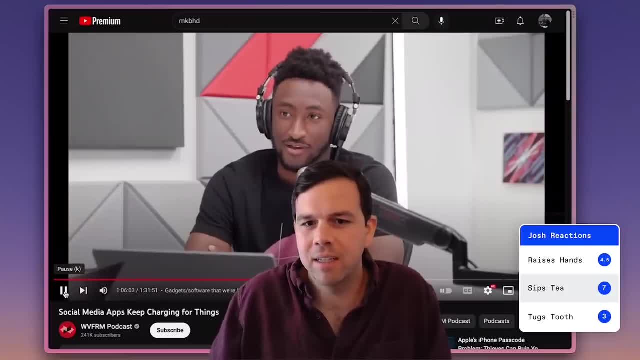 wait, do you use windows at all? no, but i need it on my phone so i can like have that sync back in the fourth, like just just having. like having the same browser everywhere is, yeah, pretty important for, yeah, bookmarks auto. i don't do that. i think they'll have the mobile version out in a couple months. 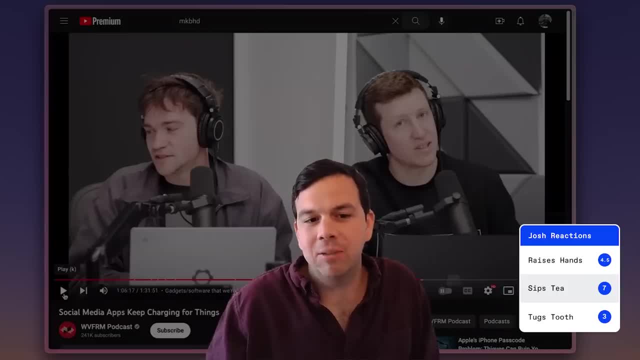 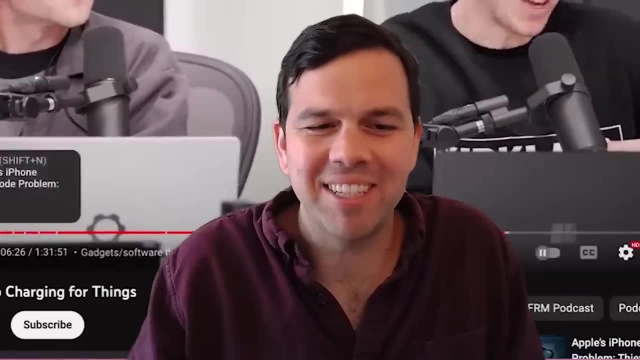 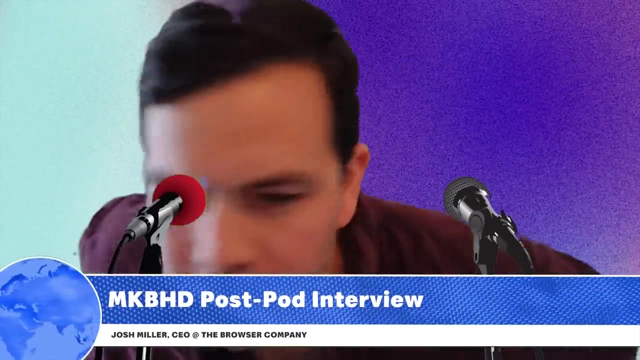 so cool. yeah, hope he doesn't use an android phone. nice cool. who wants to go? next i'm using a new smartwatch and wearing it the whole time. all right, that was awesome. just the positive energy and optimism. like i think mkbhd does a great job of being constructively. 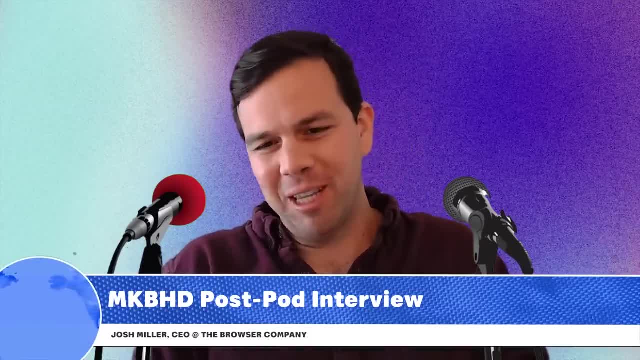 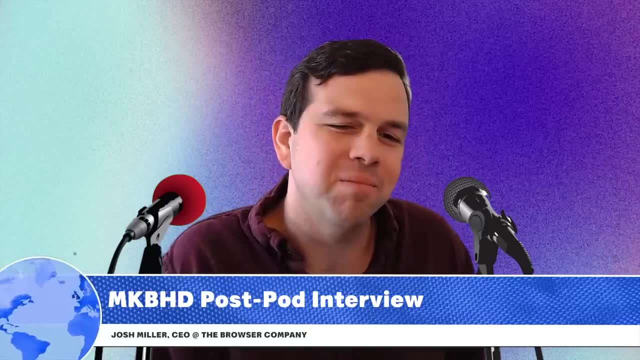 critical and honest. a large percentage of my youtube watch time is watching his stuff he puts out. but, um, as someone and as a team that's put so much heart into what we've built, just really nice to hear these folks kind of talk about it for so long. likes the name arc. that was very controversial. 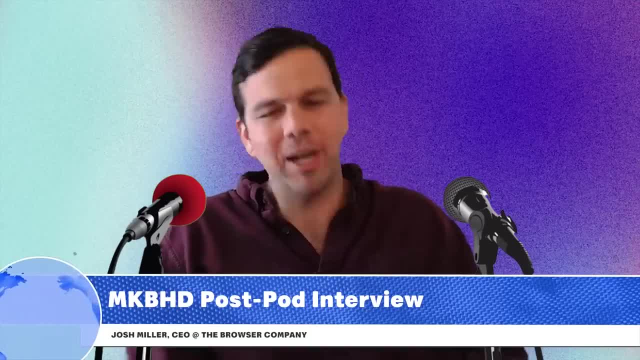 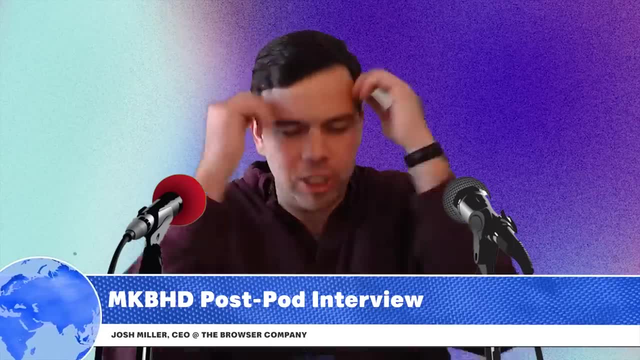 at the beginning, i'm the ceo, but i almost got fired by an insurrection at my company because i came back from a trip, wanted to name it matt m-a-t-t-e. it was just like i thought i had this. aha moment. the browser. it frames the internet. 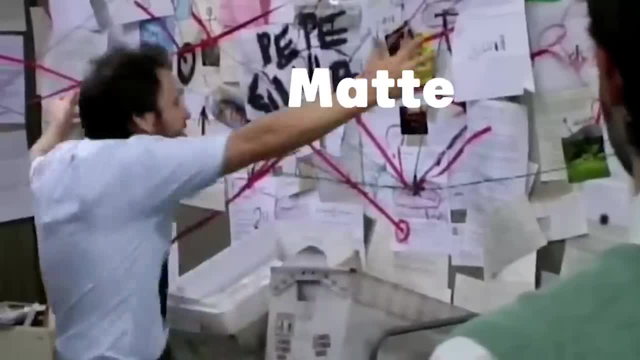 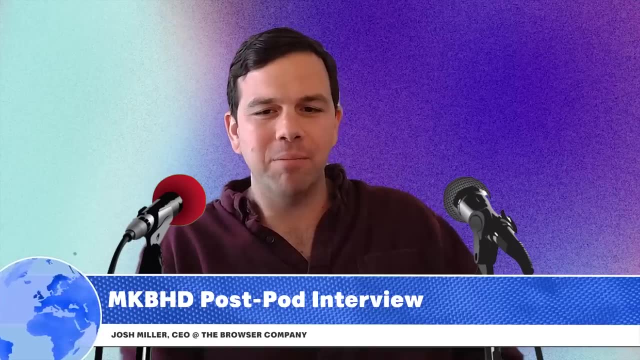 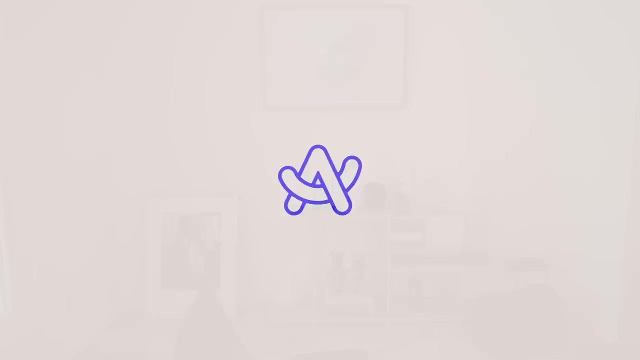 frames- man and picture frames- have mats in them. so there's one person on our team, alexandra. she's an early engineer and she didn't say she would quit if we named it matt. but she didn't not say she wouldn't quit. i'll be right back. you want to stop performing? if you want to keep it.